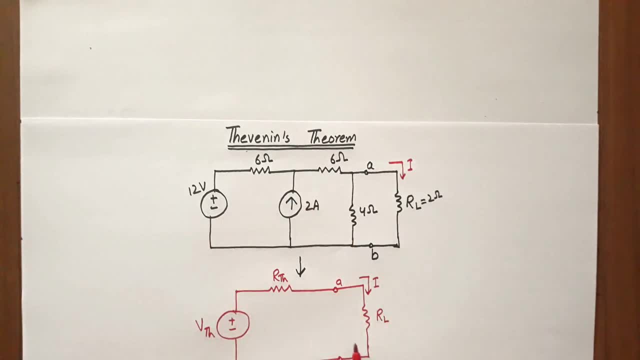 then it will be very simple to find this current. We will go through step 5.. Step 1 is that we have to find R Thevenin. That is equivalent resistance To find R Thevenin. we have some conditions That are to remove the load. 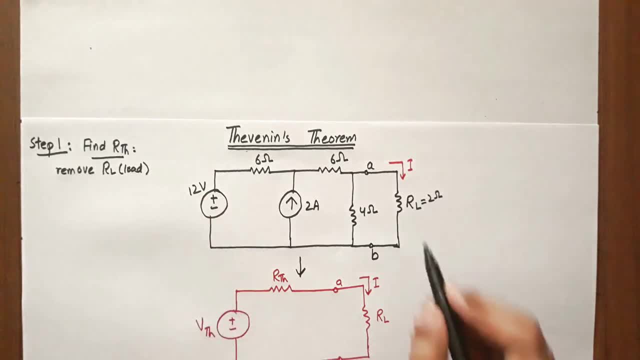 That is, to remove the load resistance RL. So if we remove it, then we have open circuit for terminals A and B- Ignore all the sources- Short circuit for voltage sources and open circuit for current sources. If we short-circuit the voltage source, then the voltage will get zero. 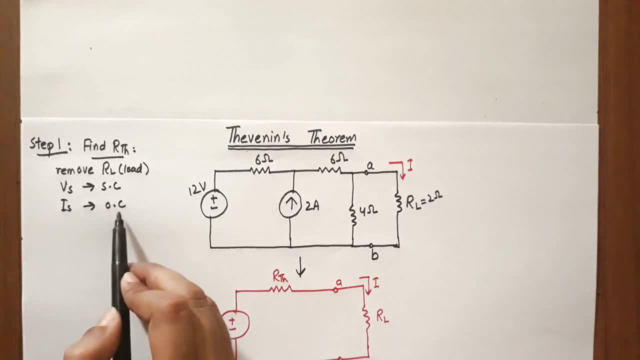 And if we open-circuit the current source, then the current will get zero. We read over the circuit with a shorted voltage, source and resistance. If the current source is open-circuit then, whether we draw it or not, It will not have a contribution. 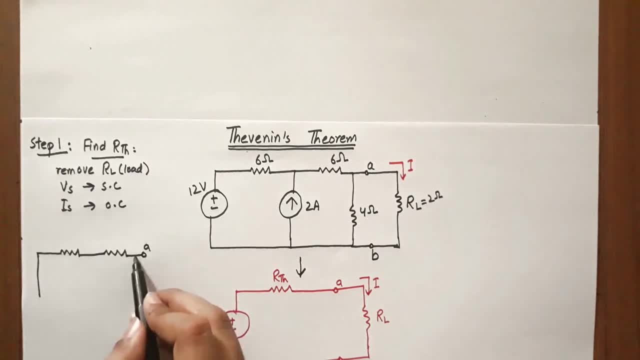 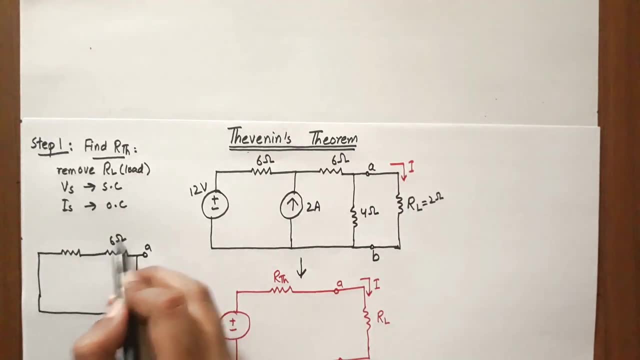 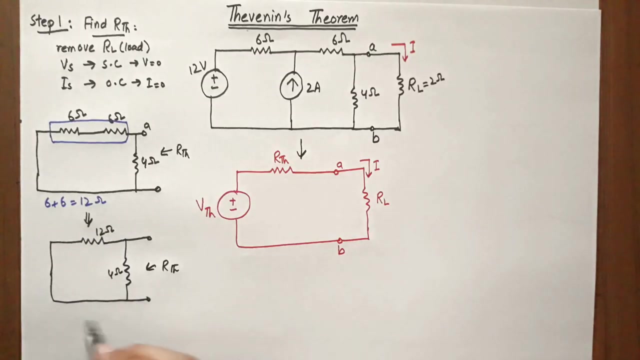 terminal A and here is 4 ohms resistance, and terminal B, V is equal to 0 and I is equal to 0, so all sources are 0. now 6 ohm resistance is in series with other 6 ohm resistance, so 6 plus 6 is 12 ohms. 12 ohm resistance is in parallel with. 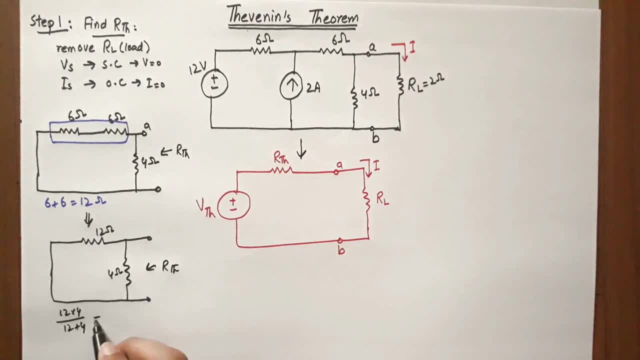 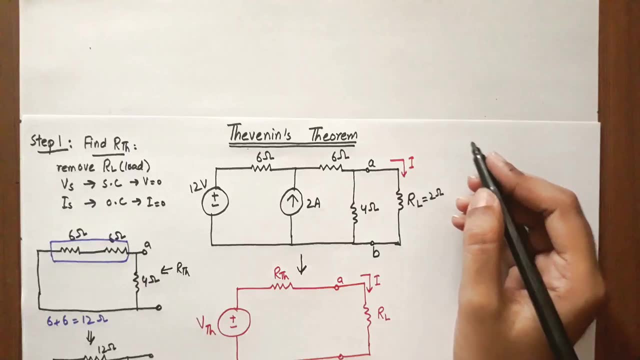 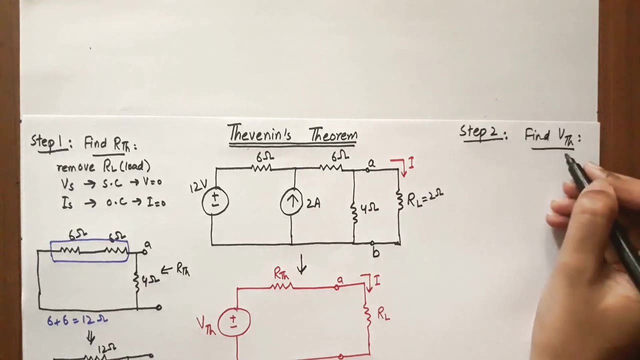 4 ohm resistance, so 3 ohms, we get one equivalent parameter, which is R Thevenin. let's go to step 2. in second step we have to find V? Thevenin, Thevenin voltage. to find V Thevenin, your load resistance, RL, we will open, circuit it or remove it, like we did for R Thevenin. 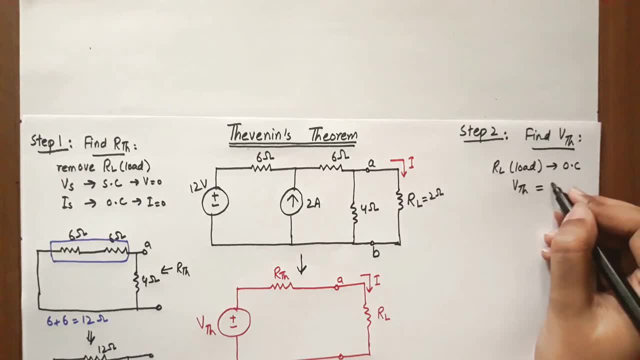 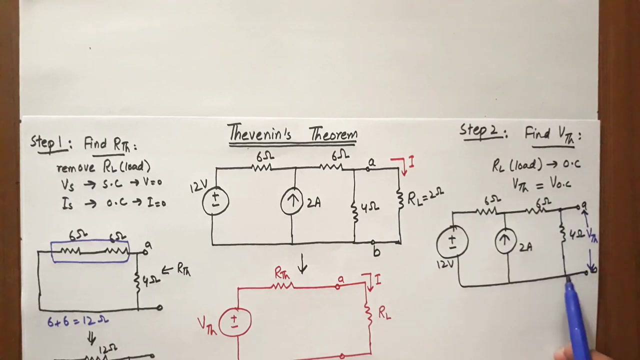 and voltage V Thevenin will be equal to that open circuit voltage. the voltage across terminals A and B is V Thevenin and V Thevenin will be equal to that voltage across 4 ohm resistance, because two are in parallel and voltage in parallel is same. 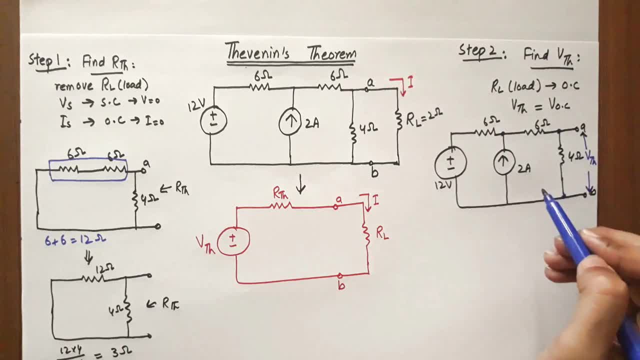 now set the voltage at these nodes. voltage is coming here of 12 volts, and on this node there is voltage V1, and on this node there is voltage V2. now V2 is across 4 ohm resistance, so V Thevenin is equal to V2. 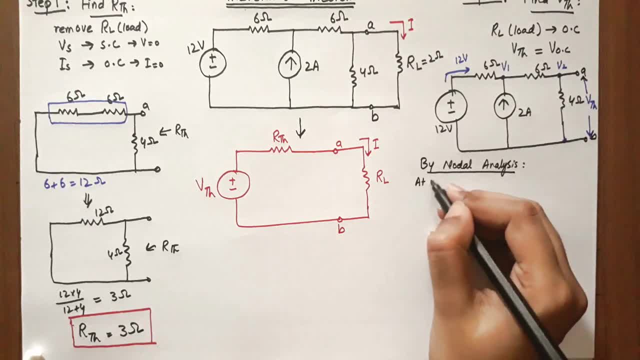 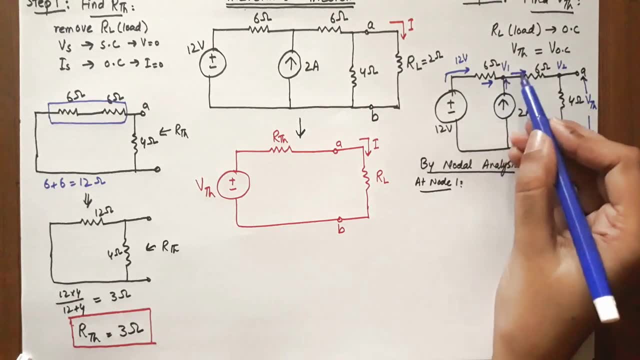 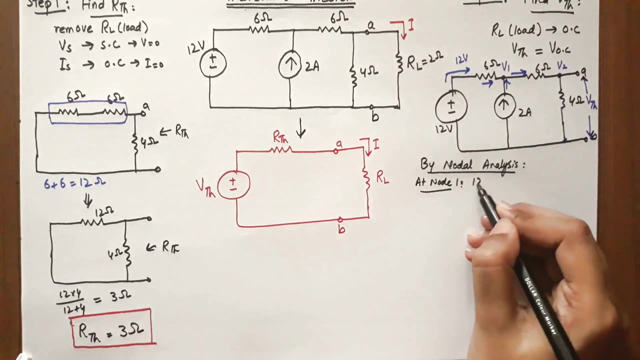 now by nodal analysis and at node 1. the voltage of node 1 is V1. current is entering here as well. these are the directions of current. current flows from positive to negative, on higher potential to lower potential. so 12 volts higher potential and minus lower potential is V1 over 6. 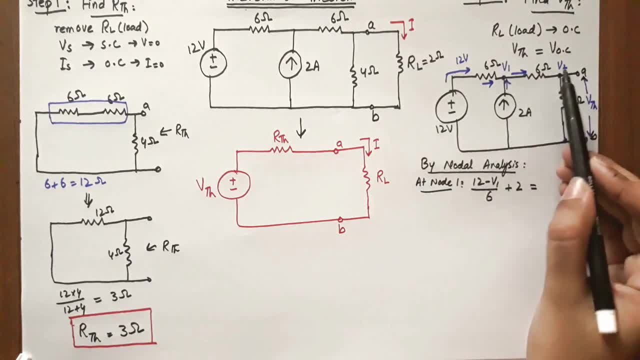 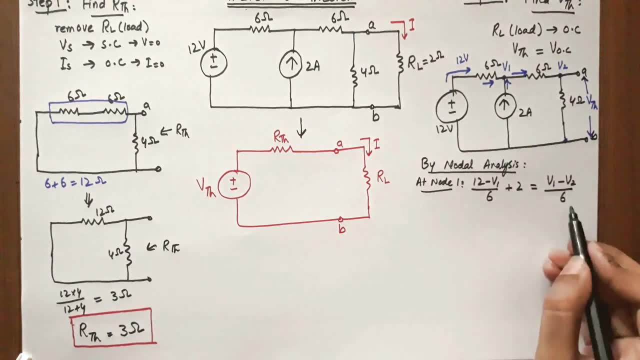 and similarly, 2 amperes is equal to V1 minus V2 over 6. so current is going from V1 to V2, current flows to V1 minus V2 over 6. so V1 is 24 plus V2 over 2. 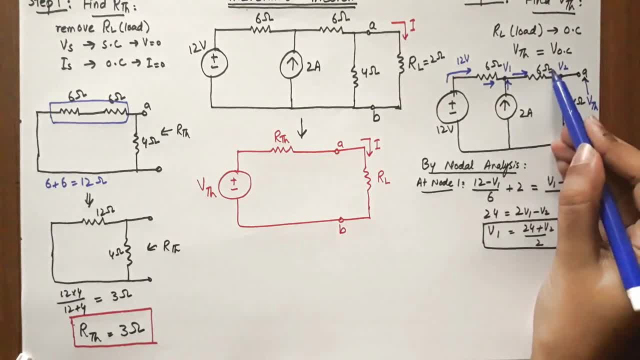 we actually need the value of V2 because V Thevenin is equal to V2. current is entering V2, after entering it will go to 4 ohm resistance and it is open circuit. so add node 2. what will happen in node 2, current is coming from 6 ohm resistance to V2. 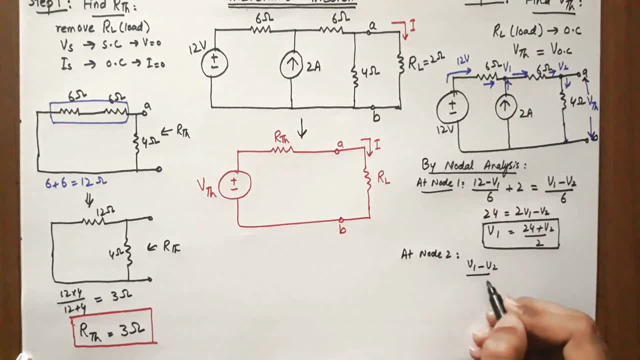 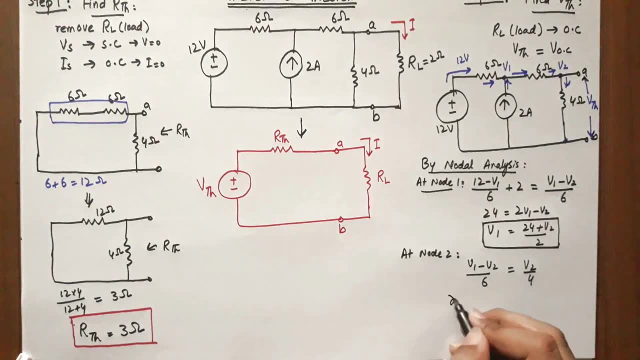 then to the second node. so V1 minus V2 over 6 is equal to V2 minus 0 over 4, V2 over 4. now simplify this equation: 2V1 minus 2V2 is equal to 3V2. now if we put the value of V1 here, then we can find the value of V2. 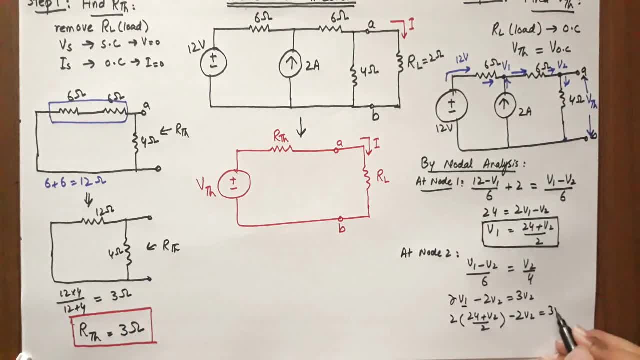 is equal to 3V2, so V2 is equal to 6 volts. so V2 is equal to 6 volts. now V2. we have said that V Thevenin is equal to V2, because V2 is parallel to V Thevenin. 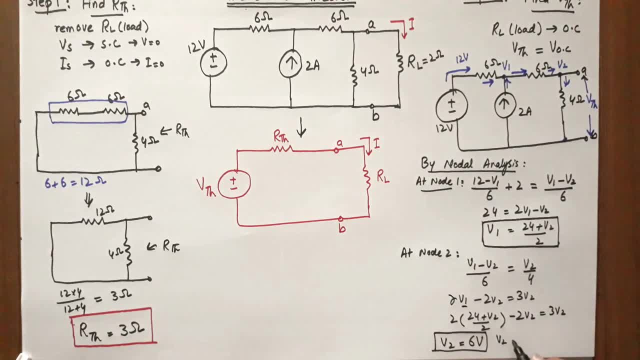 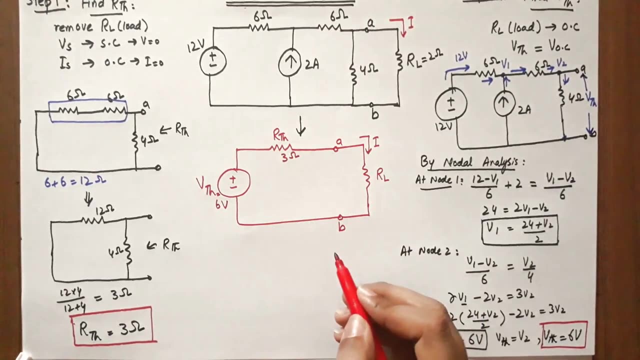 so V Thevenin. our second parameter is equal to 6 volts. so we found the two parameters V Thevenin and R Thevenin. R Thevenin is 3 ohms and we have 2 ohms. we have two resistances in circuit.